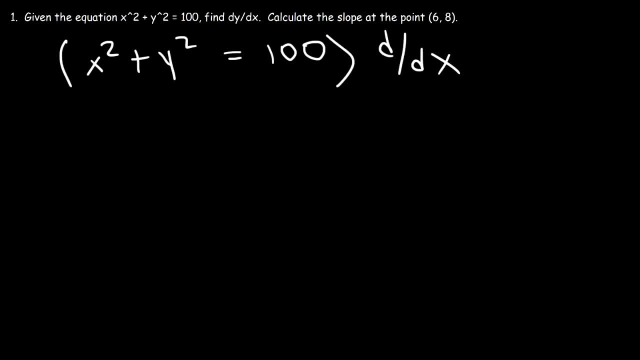 So let's go ahead and differentiate both sides. with respect to x, The derivative of x squared is 2x and the derivative of y squared with respect to x is 2y. It's 2y times dy, dx, And the derivative of a constant is 0.. 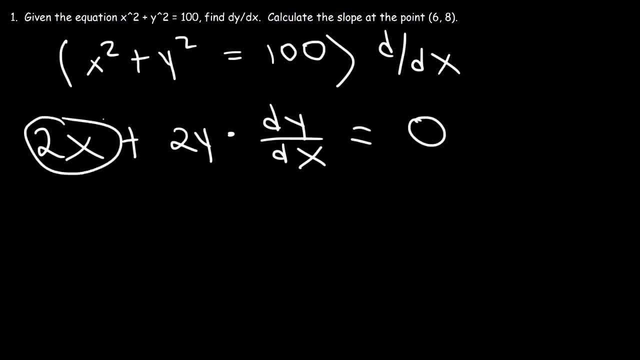 So now let's isolate dy dx. So let's take the 2x and move it to the other side. So if we subtract both sides by 2x, on the left we'll have 2y dy dx and on the right negative 2x. 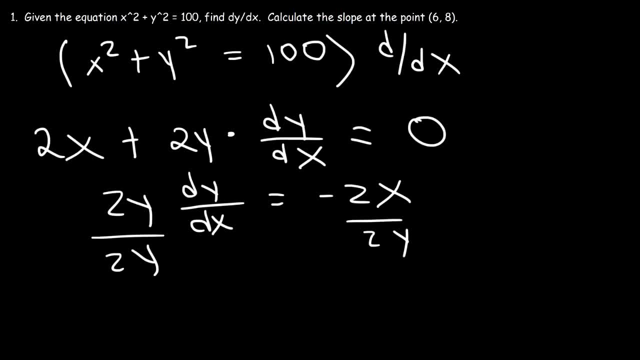 Now let's divide both sides by 2y. We could also cancel negative 2.. So dy over dx is equal to negative x over y. So now that we have dy dx, we can move on to the second part of the problem. 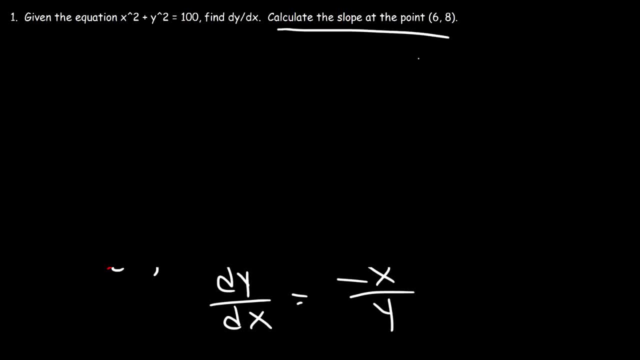 Calculate the slope at the point 6, comma 8.. So let's evaluate dy dx at that point. So x is 6 and y is 8.. So we need to reduce this fraction. 6 is 3 times 2. And 8 is 4 times 2.. 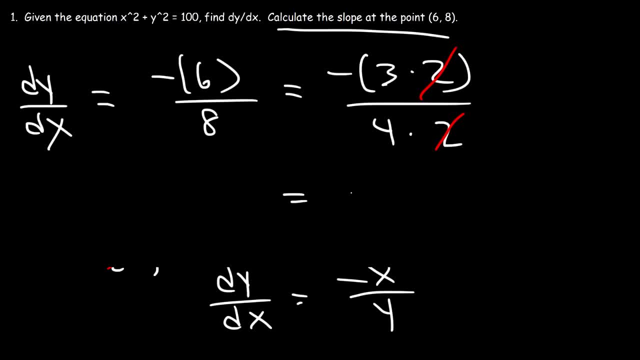 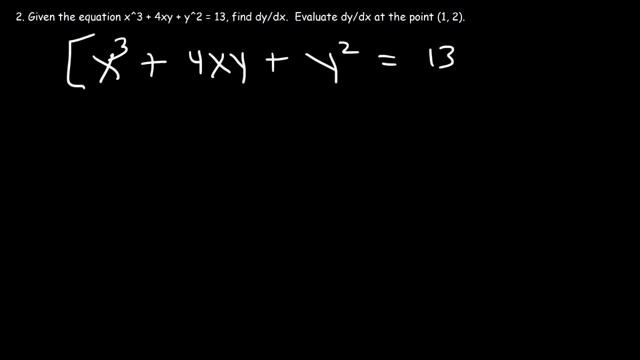 So we could cancel a 2.. And so dy dx is equal to negative 3 over 4 at the point 6, comma 8.. And that's the answer. Now let's move on to number 2.. Given the equation x cubed plus 4xy plus y squared is equal to 13,. find dy dx. 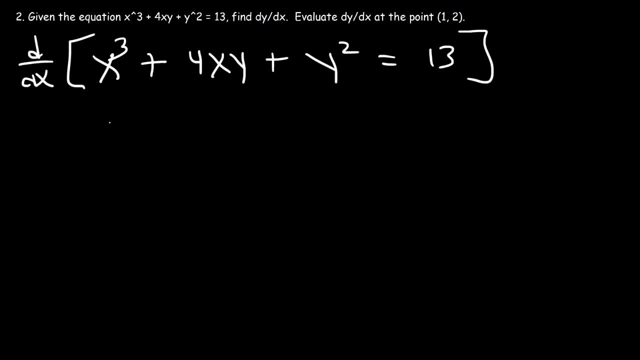 So let's differentiate everything with respect to x. So the derivative of x cubed, that's going to be 3x squared. Now what about the derivative of 4xy? Because we need to use the product rule. So let's treat 4x as if it's f and y as if it's g. 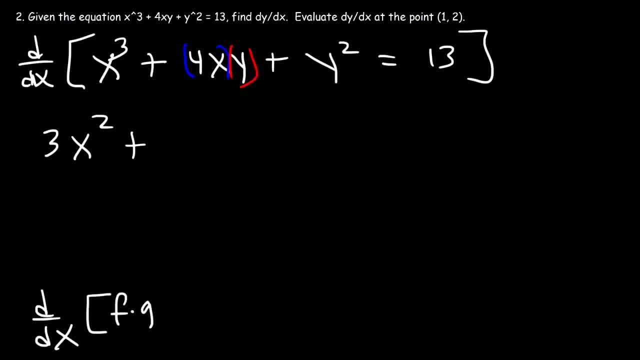 So here's the formula of the product rule. The derivative of f times g is going to be the derivative of the first part, f prime times the second Plus the first part times the derivative of the second part. So the derivative of 4x is 4, and we're going to leave the second part the way it is. that's. 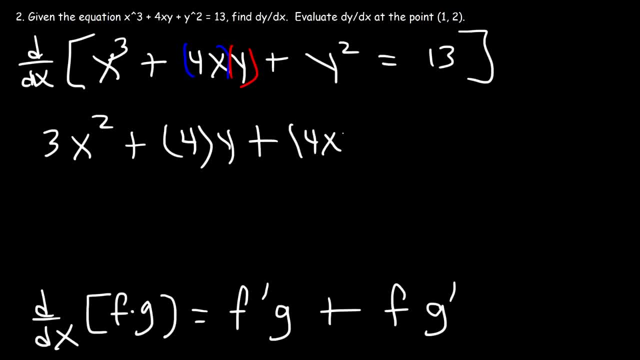 g And then plus f, the first part times g prime, the derivative of the second part, The derivative of y, is 1, but with respect to x it's going to be 1 times dy dx And the derivative of y squared is going to be 2y dy dx. 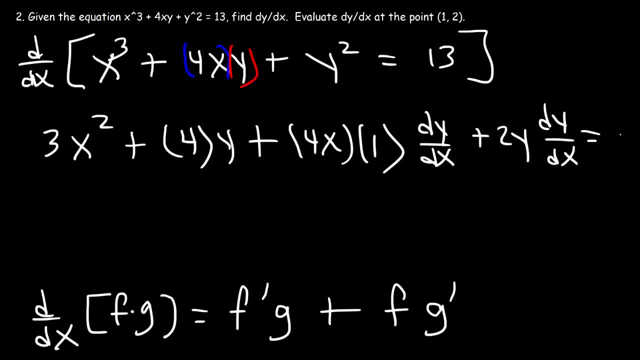 And the derivative of the constant 13 is 0.. Now we need to isolate dy dx. So what I'm going to do is, out of these two terms, I'm going to take out dy dx, So I'm going to have 4x plus 2y. 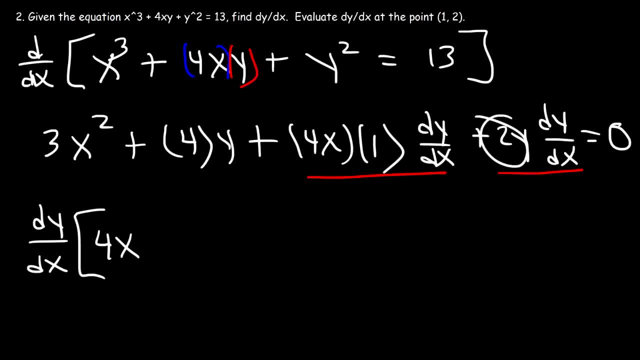 So what's the derivative of 4x? I'm going to take out 4x plus 2y. Now, what I'm going to do is I'm going to take out the derivative of 4x. So I'm going to take out the derivative of 4x. 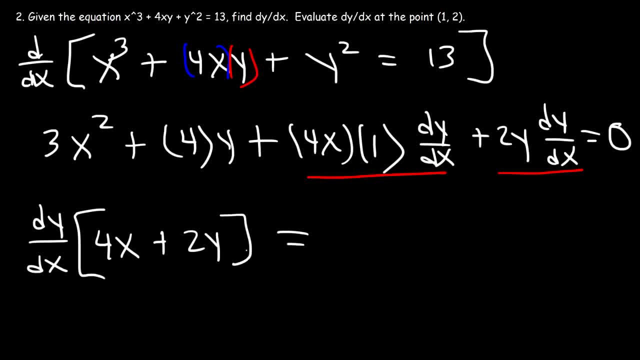 Now, every term that doesn't have a dy dx, I'm going to move it to the other side of the equation. So I'm going to move 3x squared plus 4y to the right side. They're positive on the left side, but they're going to be negative on the right side. 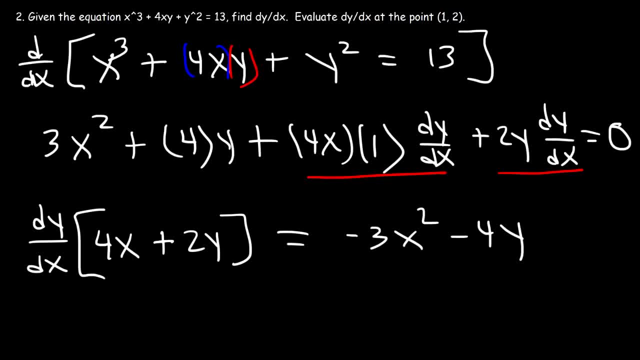 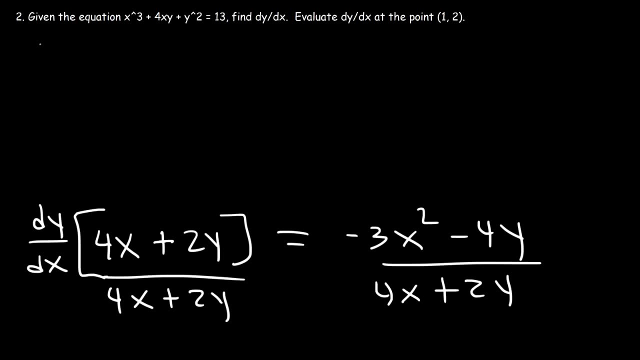 So I have negative 3x squared minus 4y. Now I need to divide both sides by 4x plus 2y, And so now I have the answer to the first part of the problem. So dy dx is equal to negative 3x squared minus 4y, divided by 4x plus 2y. 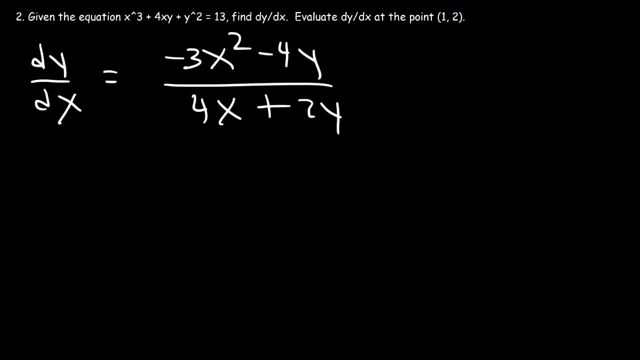 Now there's nothing else that we can do here to simplify this expression, So all we can do is evaluate it at the point. So x is 1, y is 2.. So 1 squared is 1 times negative, 3, 4 times 2 is 8, and then 2 times 2 is 4.. 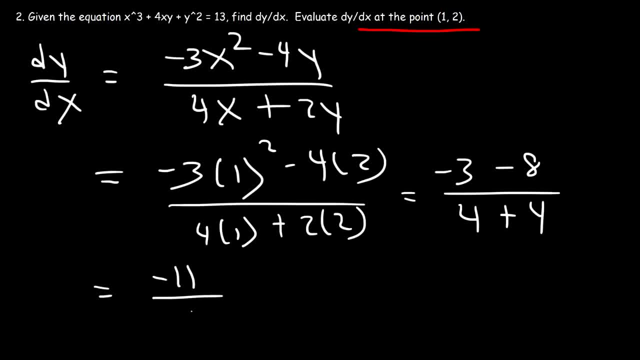 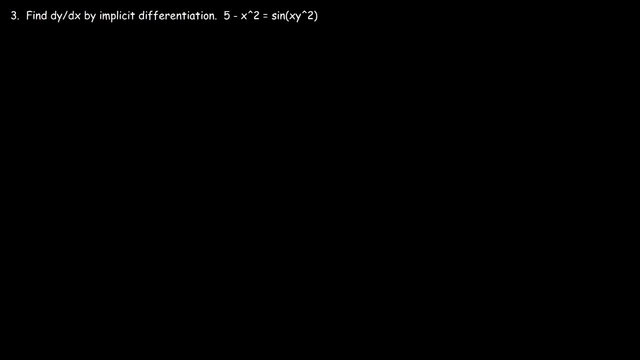 So negative 3 minus 8 is negative 11, 4 plus 4 is 8.. So dy dx is equal to negative 11 divided by 8 at the point Number 3.. Find dy dx by implicit differentiation. So let's differentiate both sides with respect to x. 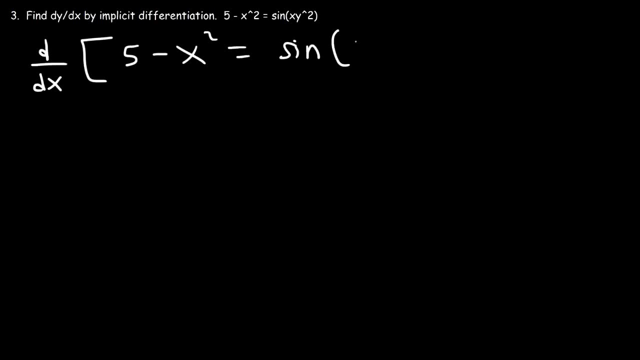 On: 5 minus x squared is equal to sin, and then xy squared. So the derivative of 5 is 0 and the derivative of negative x squared, that's negative 2x. The derivative of sin is cosine. Now, according to the chain rule, we need to keep the inside function the same. 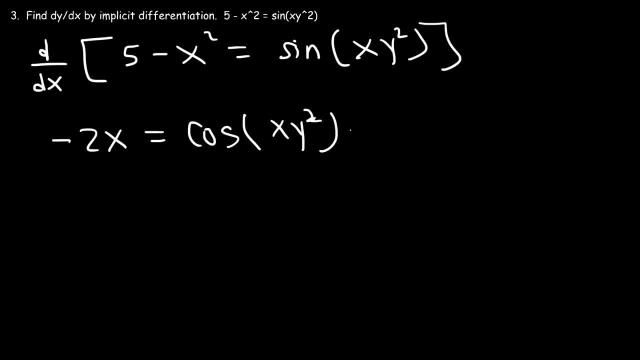 And then we need to keep the inside function the same, And then we need to keep the inside function the same, need to multiply by the derivative of the inside. So that is the derivative of x- y squared. So we need to use the product rule, So the derivative of the first part, x, is 1 times the second, y squared. 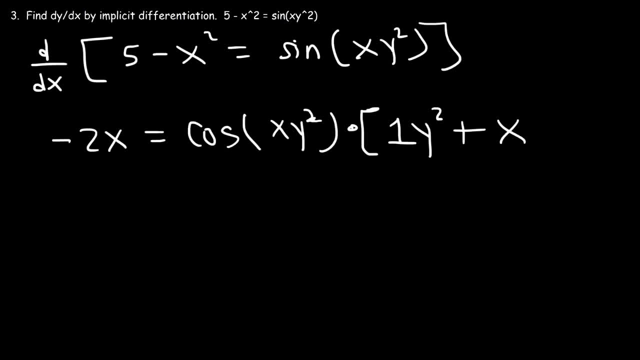 plus the first part, x times the derivative of the second part. The derivative of y squared is 2y times dy dx. So we need to isolate dy dx. Well, the first thing I'm going to do is I'm going to divide both sides by cosine: x, y squared. 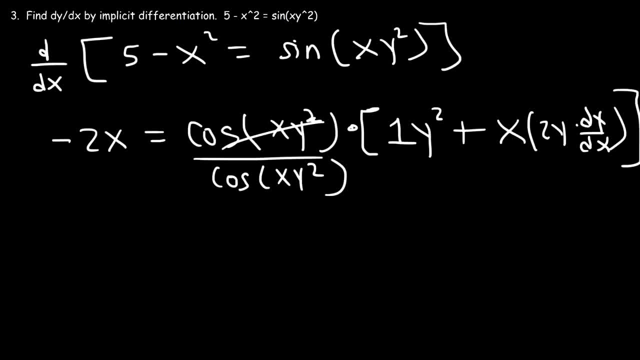 Actually, you know what I'm not going to do, that I'm going to distribute it. I'm going to distribute cosine to what I have here. So negative 2x is equal to y squared, cosine x, y squared and then plus y squared. 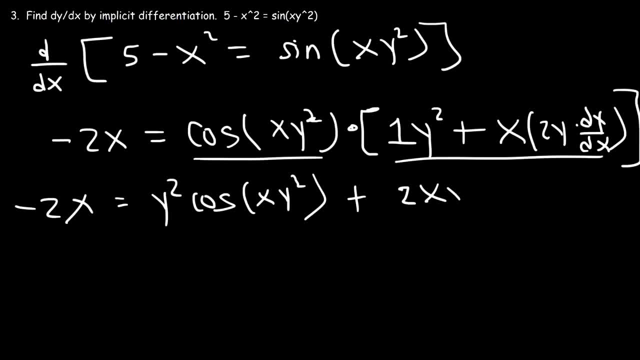 2xy cosine x, y squared times dy dx. So I'm going to take this term and move it to that side. So I have negative 2x minus this term and that's equal to 2xy cosine times dy dx. Now the last thing I 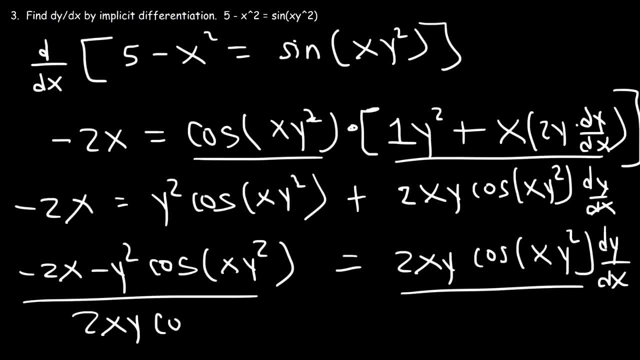 need to do is divide both sides. So I'm going to divide both sides, x and dy dx, by 2xy cosine this time over. So the final answer is negative: 2x minus y squared cosine. x- y squared divided by 2x y cosine. 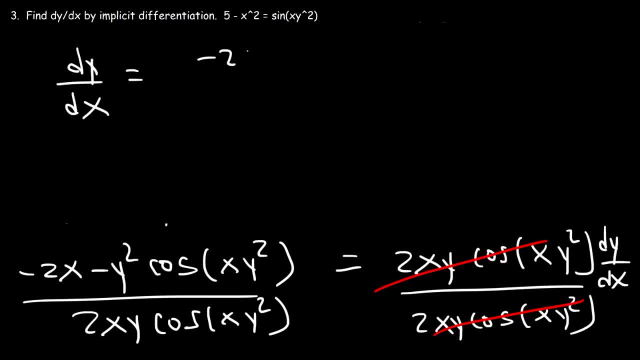 2y squared. You can substitute that with this equation, since the derivative of wanted axis is because the derivative of y squared is Q. That's the solution to this. The North Atlantic is equal to the derivative of P square by y squared. 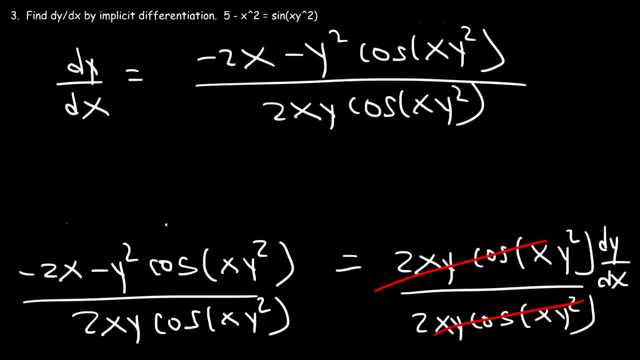 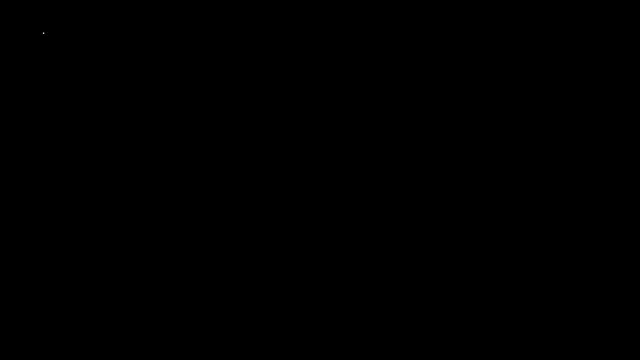 And so that's how you can use implicit differentiation with trigonometric functions. Now let's try it. one more problem. Let's say: if we have x cubed plus y, cubed is equal to, let's say, 9.. Find d squared, y over dx squared and. 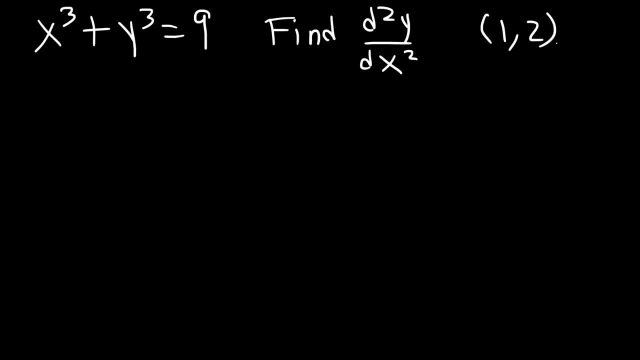 evaluate it at the point. Go ahead and try that. So first we need to find the first derivative. So let's differentiate both sides with respect to x. So the derivative of x cubed is 3x squared. The derivative of y cubed is 3y. 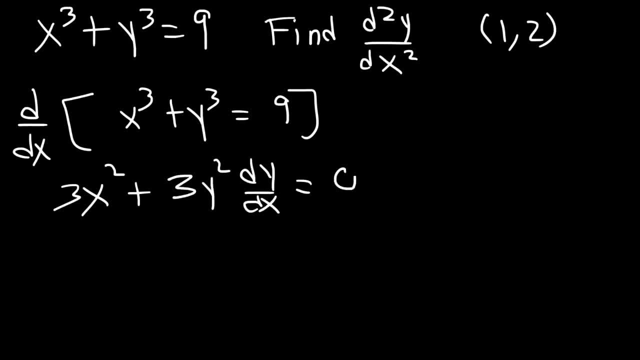 squared times, dy dx And the derivative of a constant is 0.. Now let's subtract both sides by 3x squared, So on the right side it's negative 3x squared. And then let's divide both sides by 3y squared, So dy dx is going to be negative. 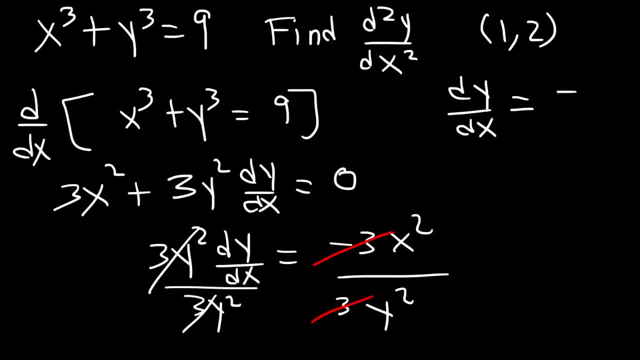 3 divided by 3 is negative: 1.. So dy dx is negative, x squared over y squared. So we have the first derivative. at this point We need to find a second derivative. So what we need to do is differentiate this function. 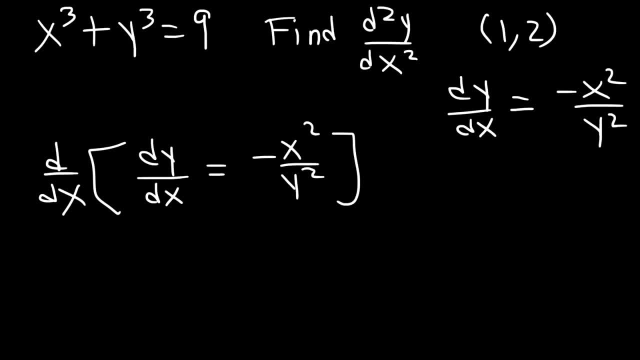 So the derivative of dy dx with respect to x is going to be d squared, y over dx squared. And then we need to use the quotient rule for negative x squared over y squared. So the derivative of f over g is going to be g, f prime minus f, g prime over g. 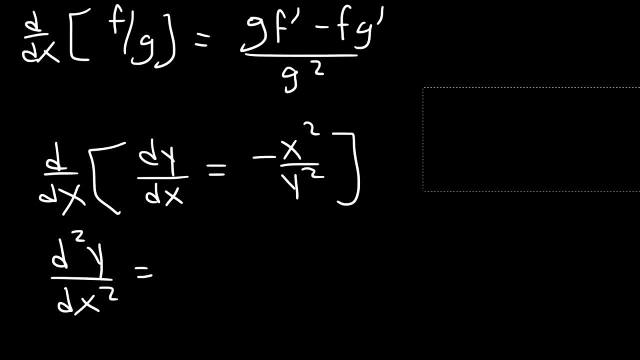 squared. So in this example, f is negative, x squared, g is y squared, So f prime is going to be negative 2x and g prime is 2y, dy, dx. So let's use this formula. So let's start with g, which is y squared times f prime, So that's negative 2x. 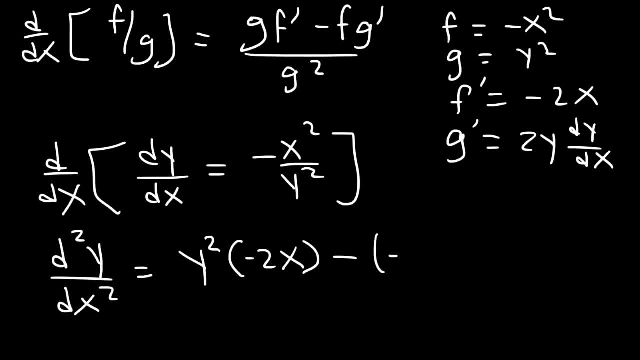 minus f, which is negative x squared times g prime. So that's 2y dy over dx, all divided by g squared, which is y squared squared. Now keep in mind dy dx is negative x squared over y squared, So we can replace that with negative x squared. 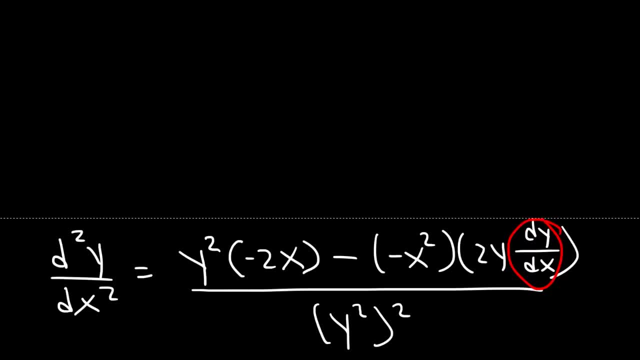 over y squared. So the second derivative is going to be: we can write this as negative 2x- y squared, and then these two negative signs will become positive. So we have plus 2x squared y, and then we're going to replace dy dx with negative x squared. 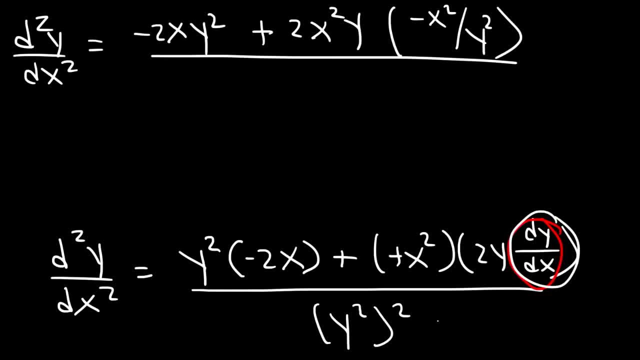 over y squared And then y squared squared is y to the fourth. At this point we could cancel a y. So we have negative 2x y squared and then 2x squared. times negative x squared, that's going to be minus 2x to the fourth power. 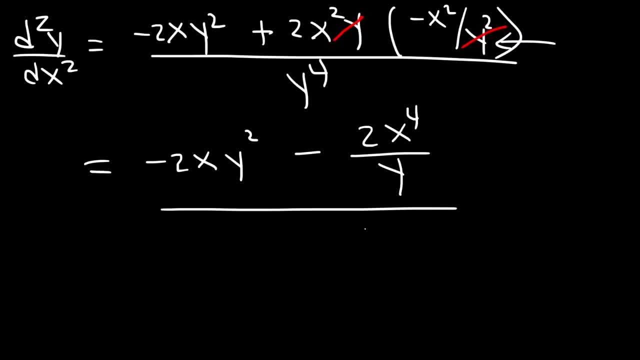 And we still have a y left over in the bottom, All divided by y to the fourth. Now to eliminate the complex fraction, let's multiply the top and the bottom by y. So we're going to have negative 2x x. y to the third minus 2x to the fourth power over y to the fifth power. 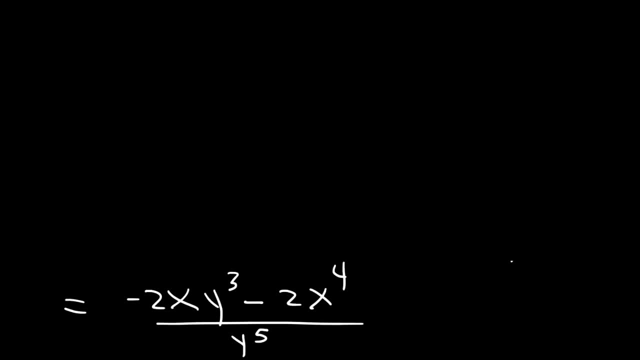 Now, if we want to, we can take out a negative 2x. So the second derivative is going to be negative 2x and then we're going to have y cubed And then, if we take out negative 2x from this term, negative 2x to the fourth divided, 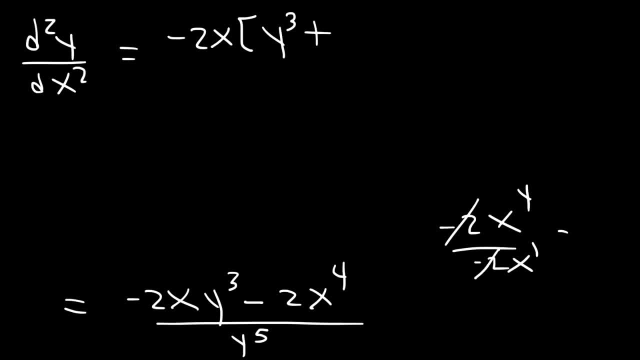 by negative 2x. the negative 2's will cancel. 4 minus 1 is 3.. So that's going to give us x, cubed all divided by y, to the fifth power. Now we have the point. So now that we have the second derivative in its